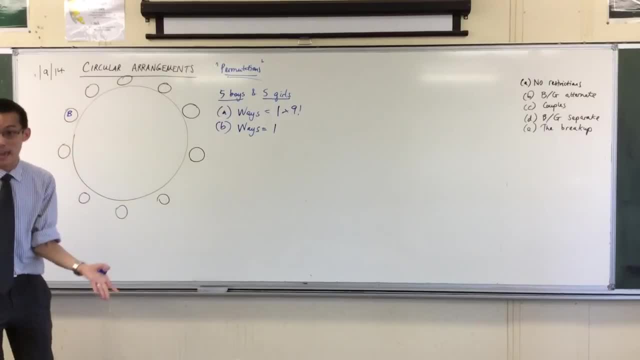 Now, don't forget, you know I put him here, but I could put him anywhere and they're all the same. So it's not like, oh, this one's different to having him over here. Same scenario. okay, Now have a look. 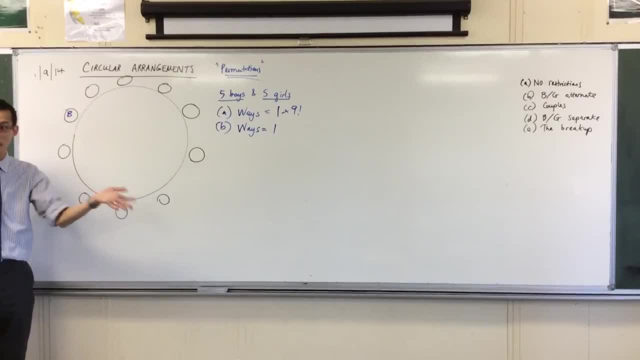 This is different to my first scenario, because now I don't just have nine people who can sit anywhere. I want to think, probably, about the rest of the boys first. I've got four boys left, okay, But they can't just sit anywhere, can they? 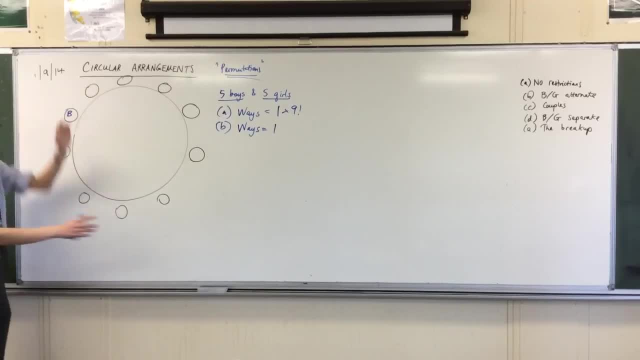 For instance, they can't sit here or here or here. You get the idea. How many places can they sit in? And the answer is: there are four potential spots left, namely here, here, here and here. okay, So now I have four spots and four boys to fill them with. 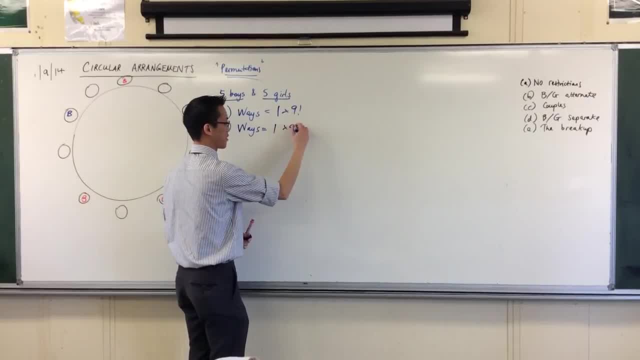 So how many ways can I do that? Four factorial, okay. And then the girls come along, five spots, five girls to fill them with Five factorial Simple stuff, okay, Alright, let's see What if? what if everyone has a partner? 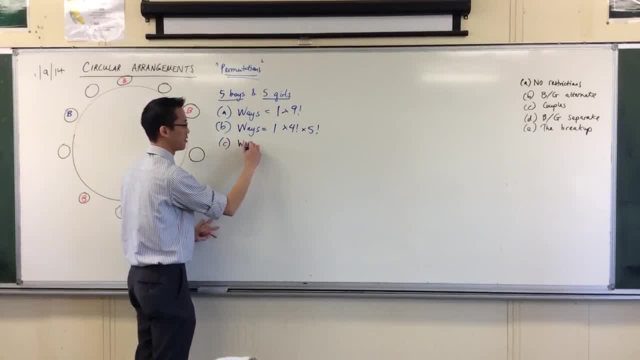 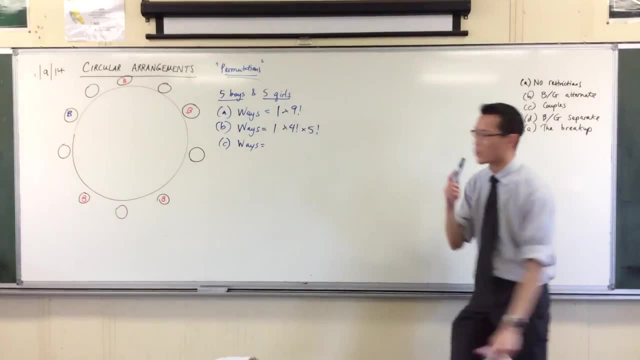 Boys and girls are all matched up and they want to sit together. okay, So they're all in couples right Now. you can think about this a couple of different ways. You can think: hmm, okay, I'm going to place someone first and then there'll have to be a specific. you know, place a boy. 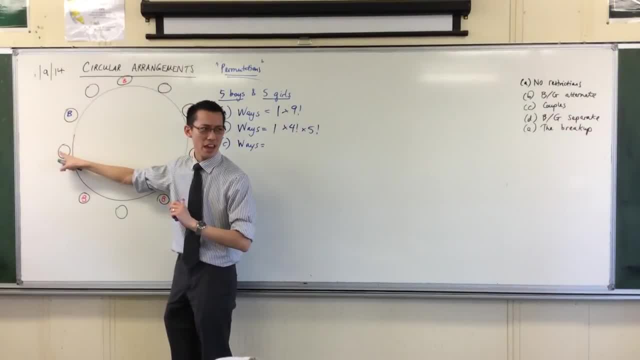 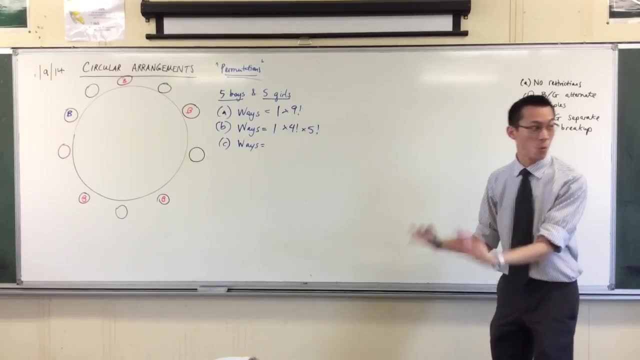 Then there'll have to be a specific girl next to them, And then I've got to place a boy, Then I've got to place another, But it starts to get confusing very fast, okay, So how can we think about this in a better way? that will make this kind of step really easy, right? 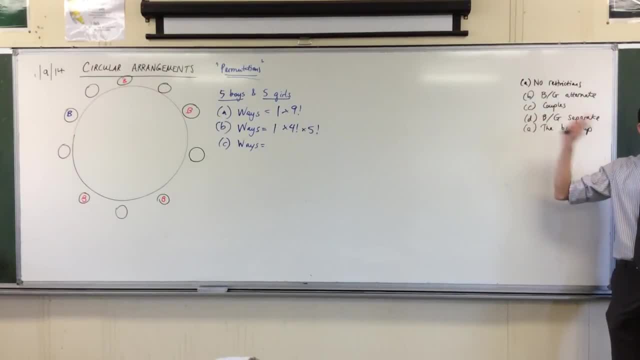 Well, think about it like this: There are five couples, right, Five couples, And, as anyone who has friends who are couples knows, sometimes it can be very hard to pull couples apart. In fact, with this situation, they are practically inseparable. 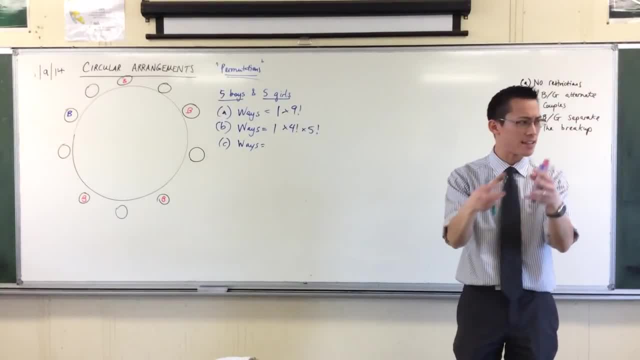 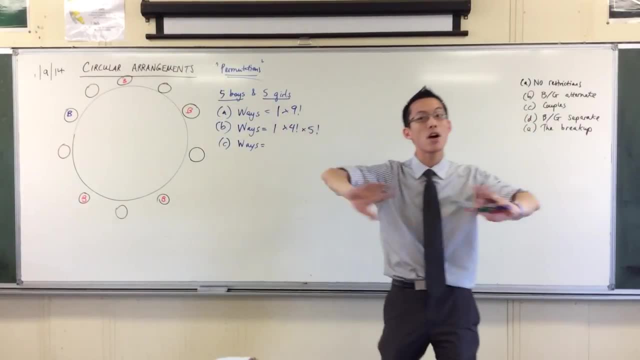 You actually can't take them apart, right? So they really function as singles. They're like little units, right? Each couple is a unit, okay? So therefore, you no longer have five boys and five girls that you can think of separately. 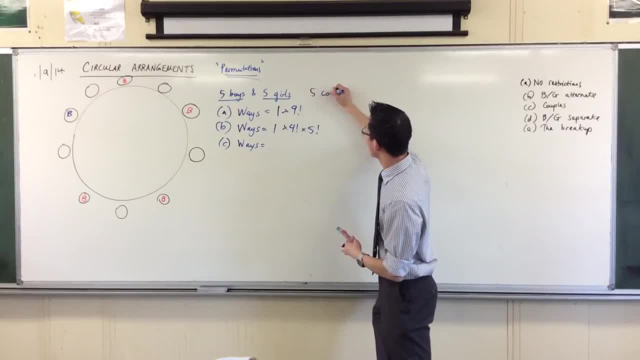 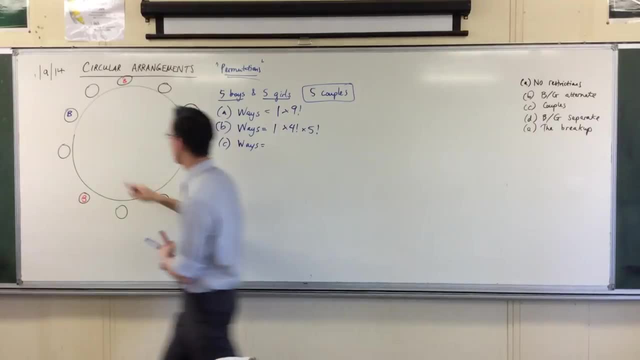 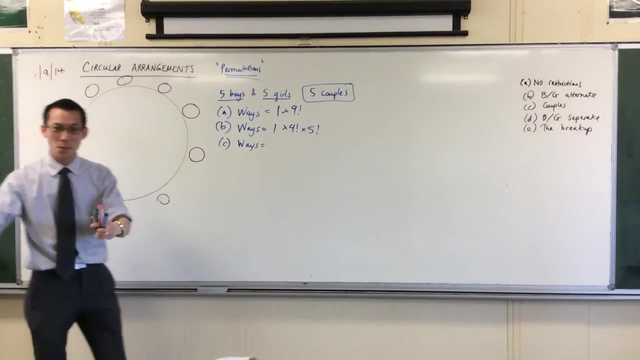 What you really have is five couples. This is the unit that I'm going to place, okay, So now let me divide up, Let me get rid of these boys for a second. Okay, Your first couple walks up right, Arm in arm. okay, 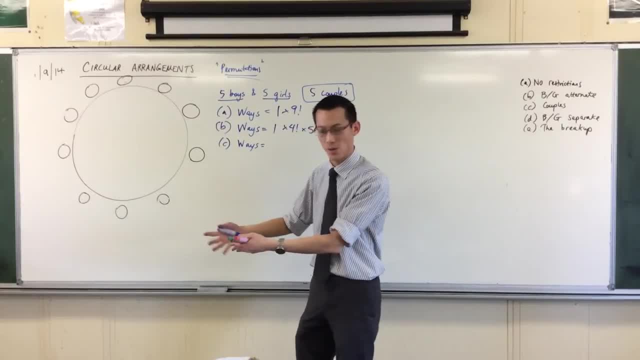 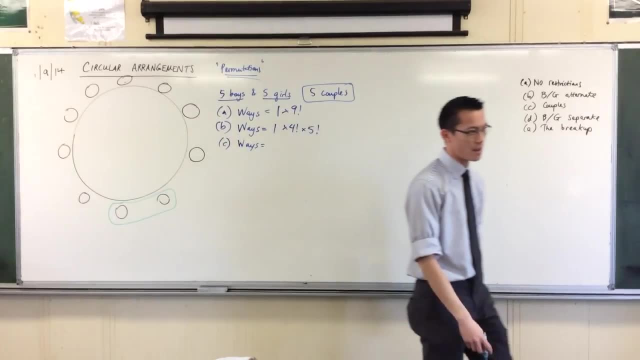 And clearly they're going to sit together. They're going to occupy seats that are next to each other, right? So, for instance, I'm going to place them here. There's a couple, okay, Now think The next couple that comes along, right? 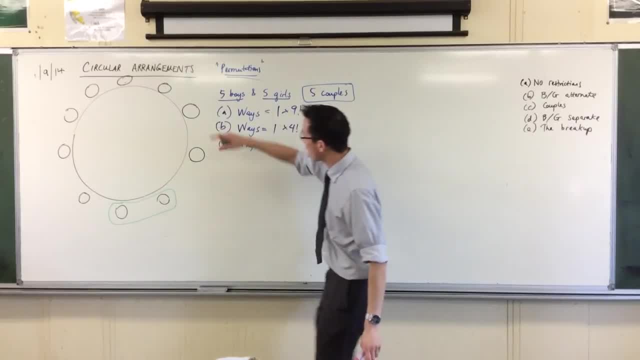 Because all the couples have to sit together. a couple can't sit in these spots over here. Can you see that? Can you see why? Because then there will be something that will break the whole couple arrangement right. So therefore, the next couple arrangement only has a few spots they can sit in. 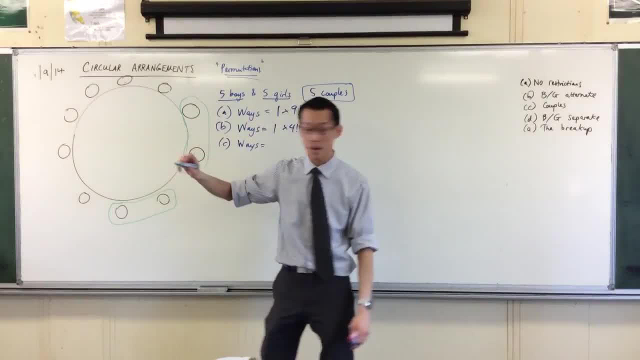 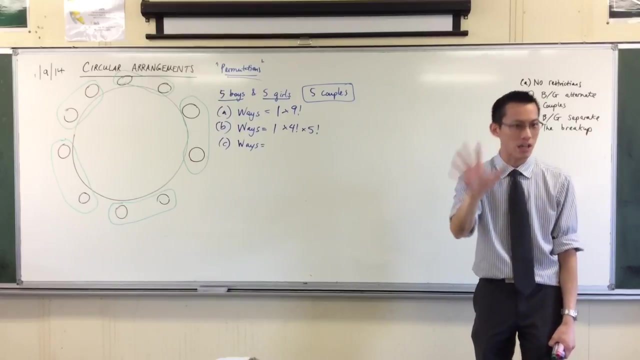 They could sit here. There's a potential spot, Or they could sit here, Or you're starting to get the point, okay, So what I have is not really a table with ten chairs. Actually, I have a table with five slots for couples. 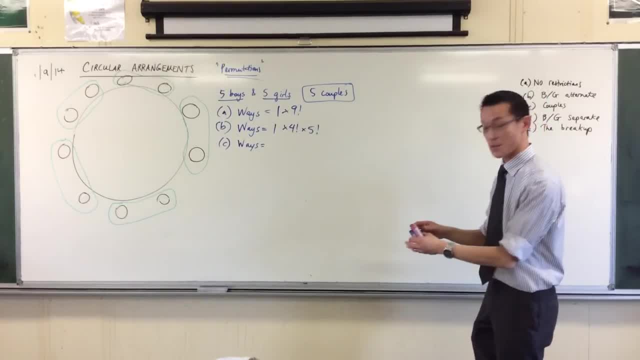 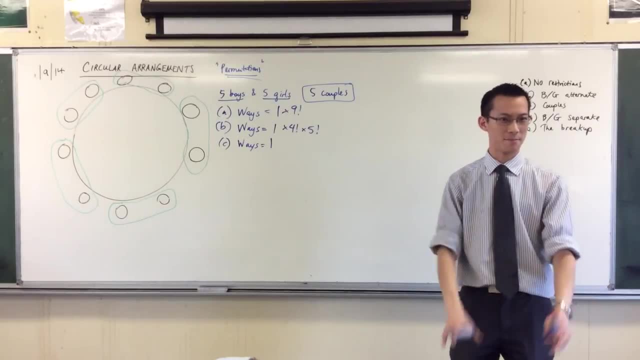 Does that make sense? Five slots for couples, okay. So here's what I'm going to do. I'm going to place the first couple- Now- I don't have to worry about the circular spinning around rotating thing, okay. And then I have to place the other four couples. 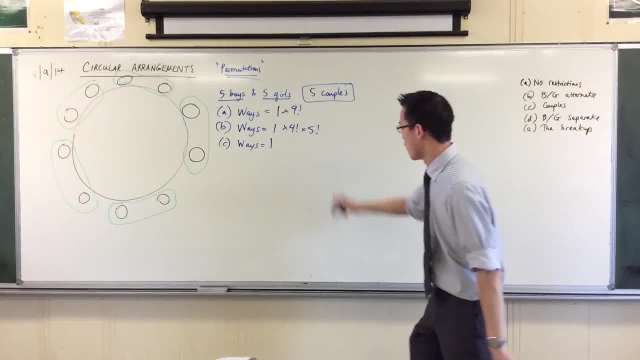 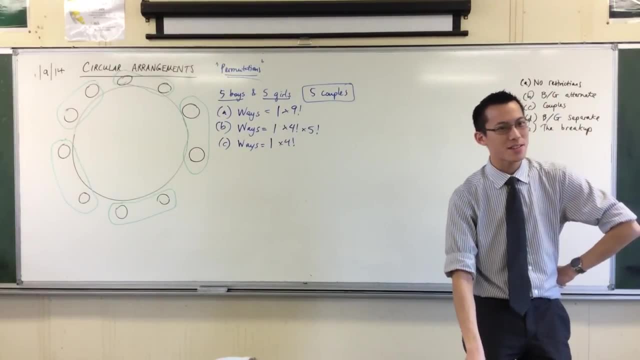 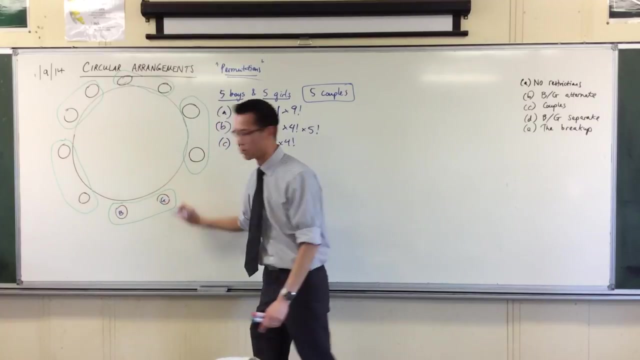 How many ways are there to arrange four couples? Four factorial, Okay, But then of course, there are more arrangements than this right, Because, for instance, let's have a look at that first couple who we placed right- The boy could sit on the left and the girl could sit on the right. 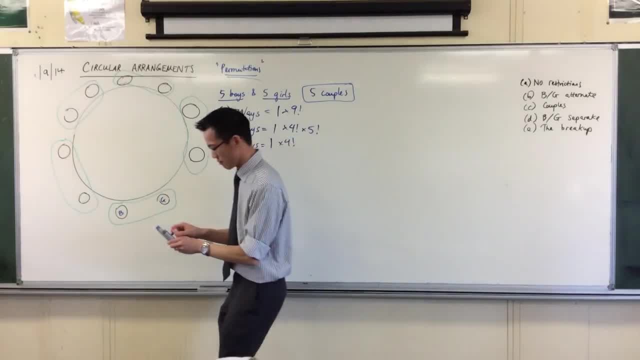 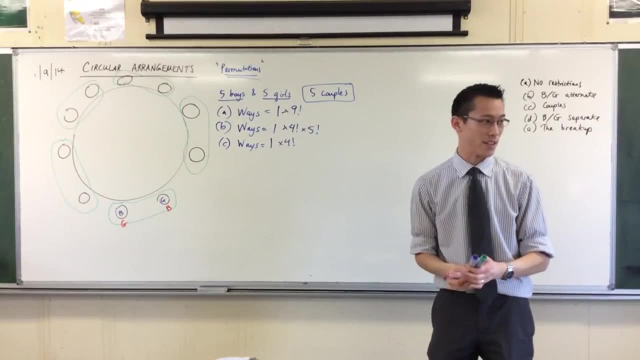 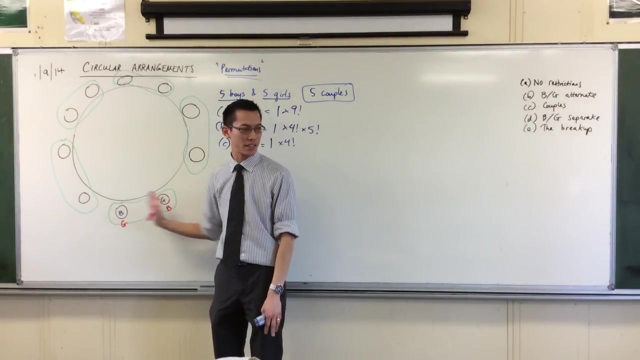 Or they could switch. okay, Now, not only can that first couple switch, they can all switch And there's no problems, right? So here I have. how many ways can I do the boy and the girl together And it's a two factorial right? 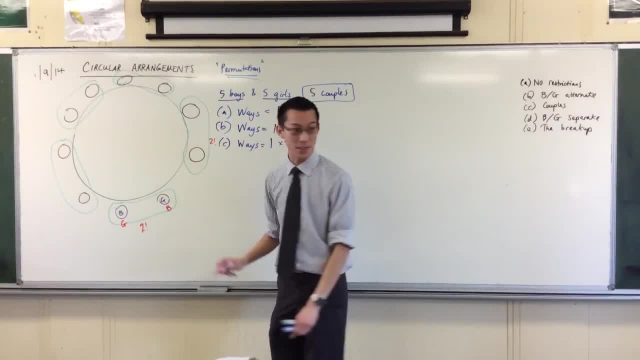 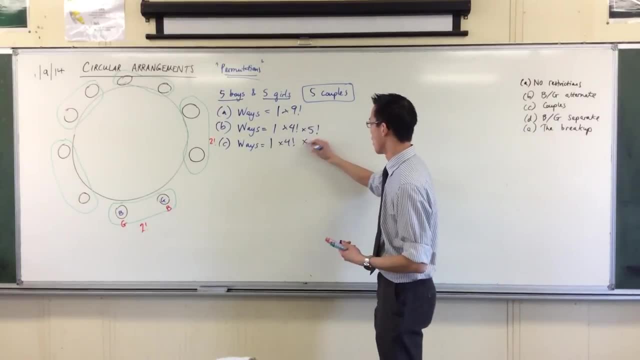 Two factorial ways for that couple and two factorial ways for this couple, And you're starting to get the idea right. So, in fact, I have undercounted by a factor of two factorial, which is just two to the power of. well, how many couples are there?